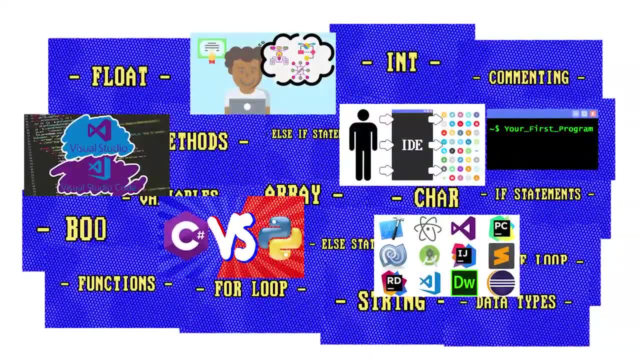 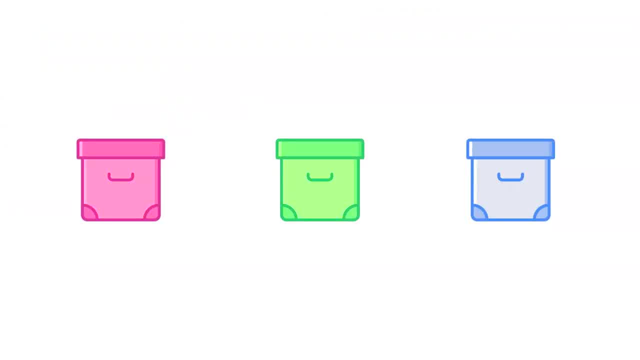 these in particular. I have a lesson on each and every one of them. Check the link in the description, because this lesson will only briefly go over them Now. again, every single one of these have their own unique set of rules and instructions. For instance, let's take a look at the integer data type, which are a type of data for whole. 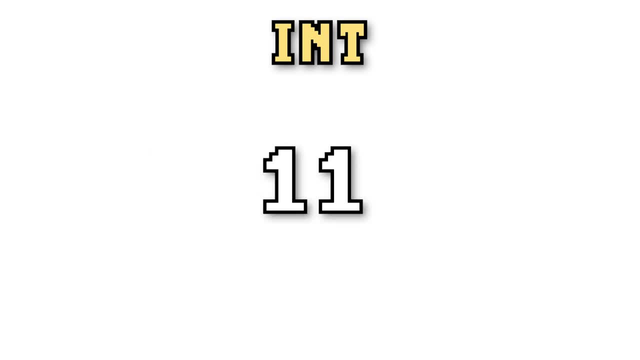 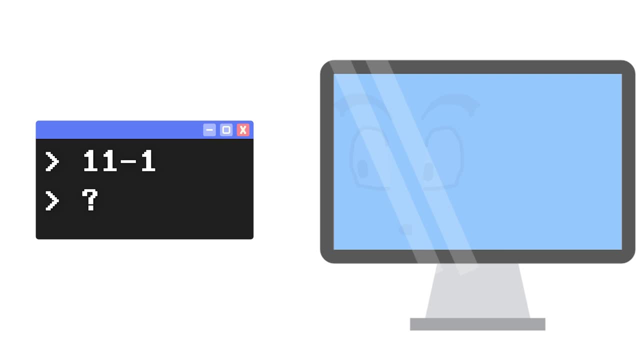 numbers. Let's say that you have an integer that equals 11, and you want to minus 1 from the integer 1.. Well, you'd write off this operation, send it to the computer to perform, and guess what? Your computer would take a look at this operation then will look to. 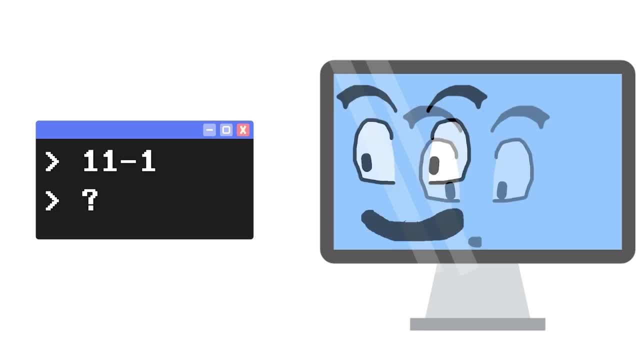 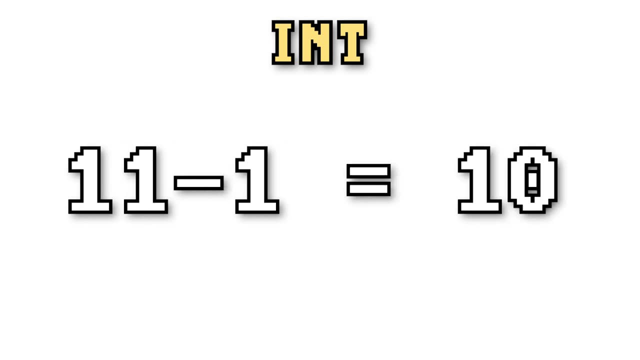 see if it has the instructions for doing that operation, Then will go. yeah, I know how to subtract an integer from an integer. The computer will then subtract 1 from 11, and then send back to you a 10.. All well and good, everything checks out. 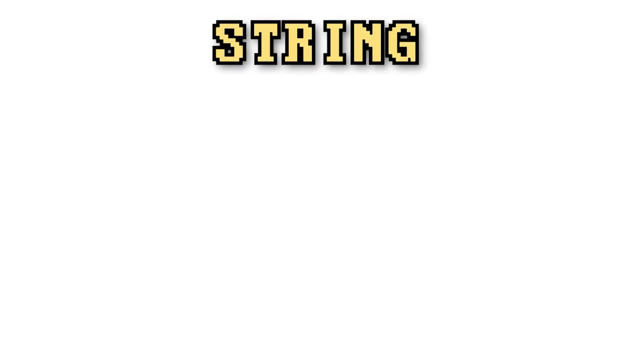 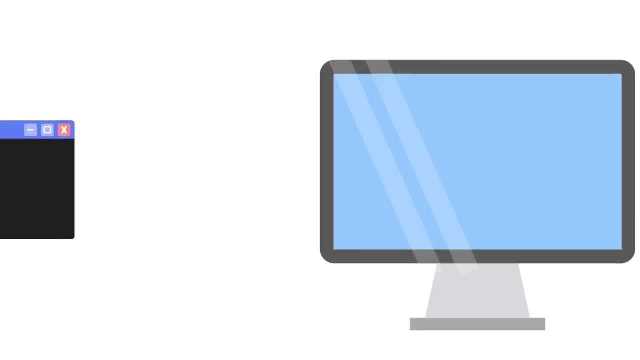 But now let's take a look at a string data type, which again is a string of characters. If you were to have the string 11, and you wanted to subtract the integer 1 from the string 11,, well, you'd send this operation to your computer. Your computer would take. 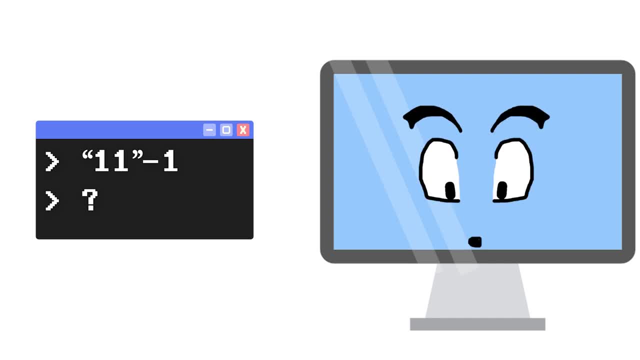 a look at this operation, then check to see if it has instructions on how to do that or not. Then it would realize what you sent. it makes absolutely no sense. It has no instructions on how to subtract integers from strings. This is no difference from telling your computer. 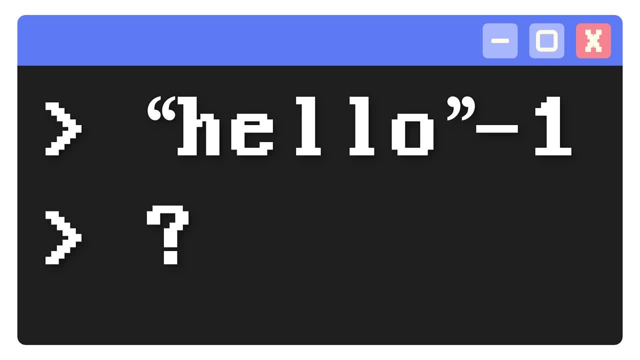 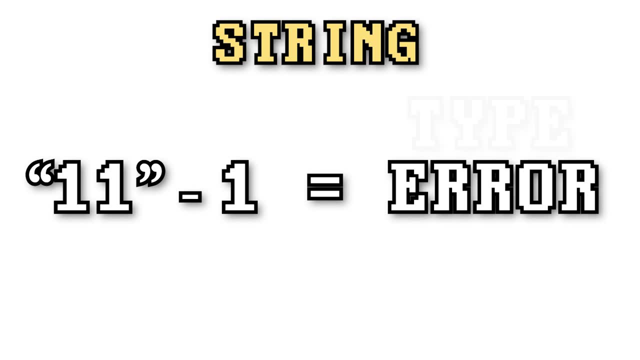 to subtract 1 from the word hello. How do you do that? So your computer will just send back to an error letting you know that the operation you are trying to do makes no sense. The next part is a type error. Now let's do the same operation, but instead make both. 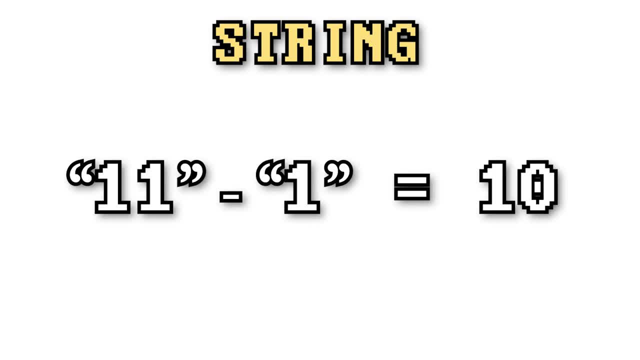 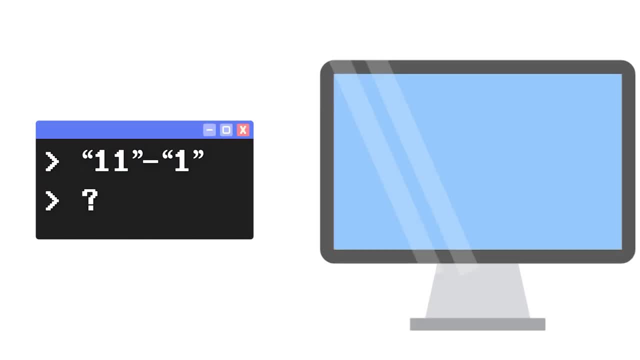 of them strings. What do you think will happen? Will we get a 10 again, but as a string? Maybe we'll get another error. Well, if you again have the string 11, and you send the operation to your computer to subtract the string 1 from the string 11,, your computer will look: 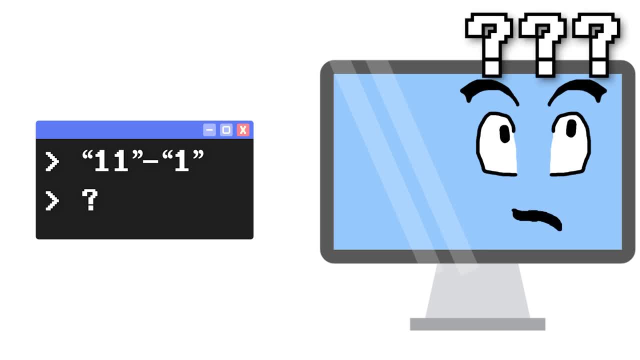 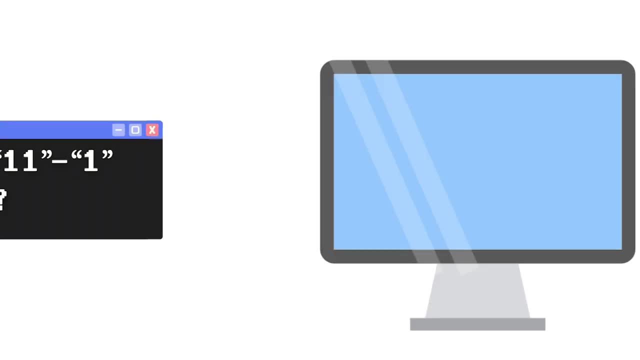 at this operation, then again realize it has no instructions on how to do this, thus returning back to you an error. But you may find this next part quite interesting If you instead tell your computer to take the string 11, and plus the string 1 to it. it.